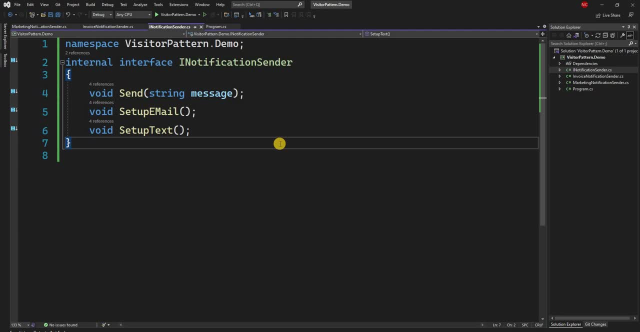 situation where we have a notification sender. Now notification can be any type of notification, A notification about an invoice or a marketing material or a subscription getting expired, because all of them will have different content as well as different logic which will trigger them. Now, for the notification itself, it is just a single method send, But the notification can. 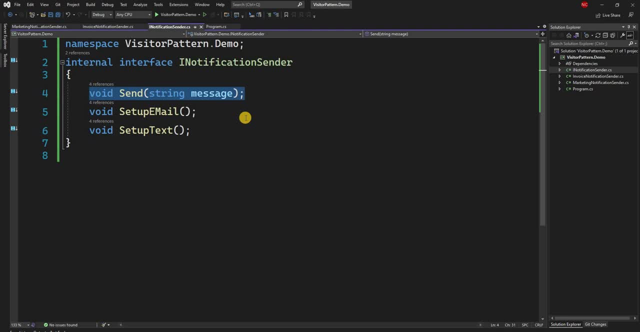 be sent through multiple mediums. It can be sent through an email, it can be sent through a text. So initially, when we built the system, we decided, okay, we are going to have two modes of notification, which is email and text. So we created our interface such a way that it sends. 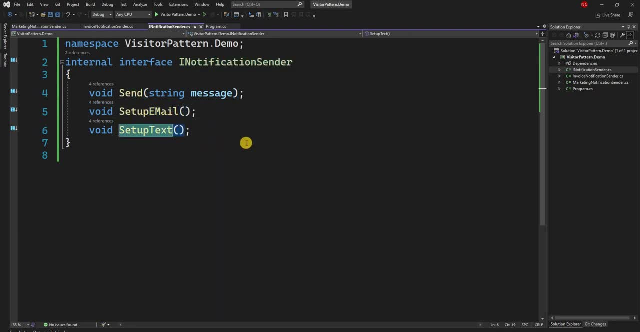 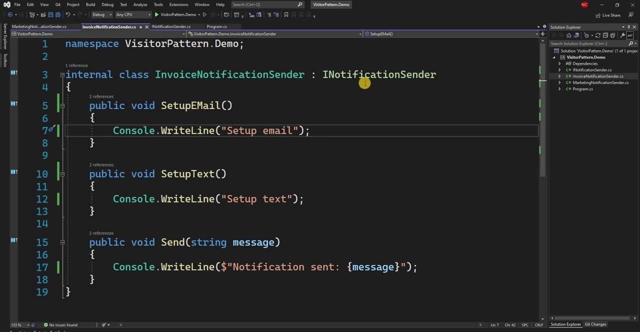 the notification and then it allows to set up the email and text notification type. And then we have a invoice notification sender which goes ahead and implements the notification sender and provides implementation of setup email, setup text and send. Right now I'm just doing a consolewriteline. 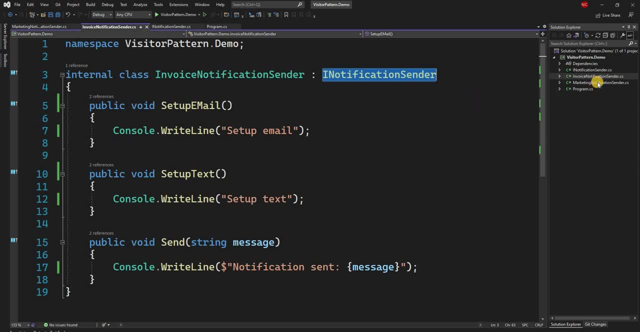 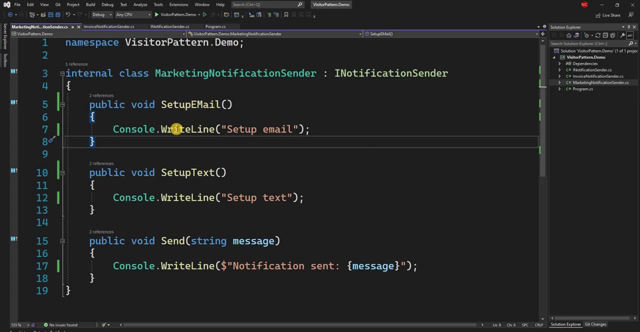 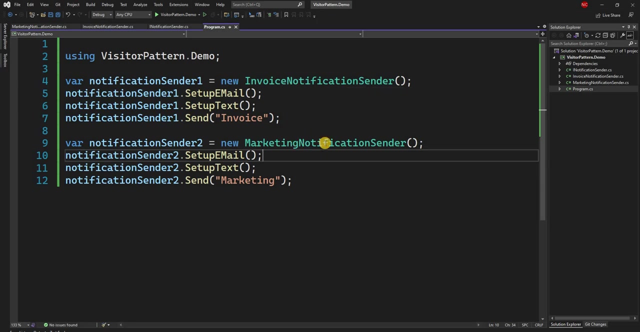 but this gives you an idea how the current implementation is done. And similarly we have a marketing notification sender, which also implements the inotification sender, and it does the same thing. It sets up an email, sets up a text and send a message And then in program class we create the invoice notification sender- marketing notification. 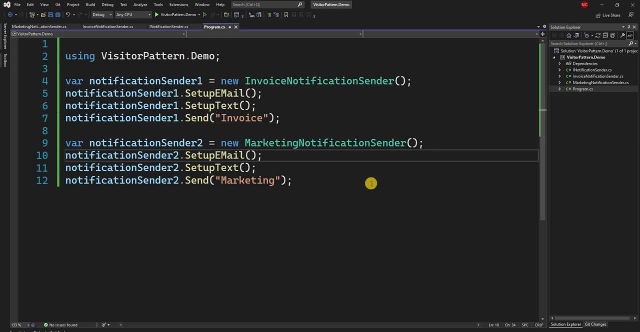 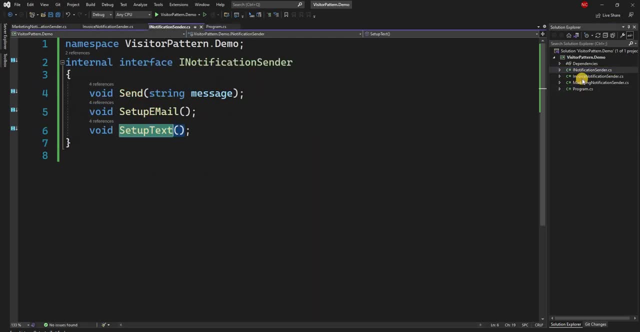 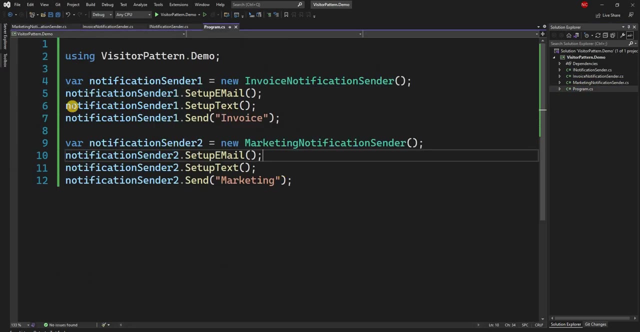 sender. We set up both email and text for both of them and then send a message. Now, at a first look, this implementation doesn't look so bad. It has an interface and then individual classes implements individual types of notification sender And then you can use them to send notification. You can. 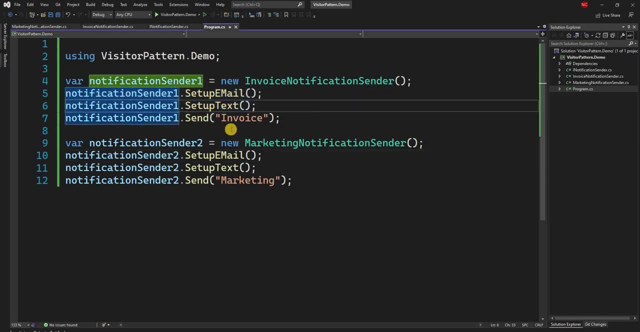 also use either email or text, based on what setup you call here. Now, of course, if you are using solid design principles, this implementation will be a little bit different, But let's keep focus on the gang of four design patterns and visitor design pattern. So now let's just run this application. 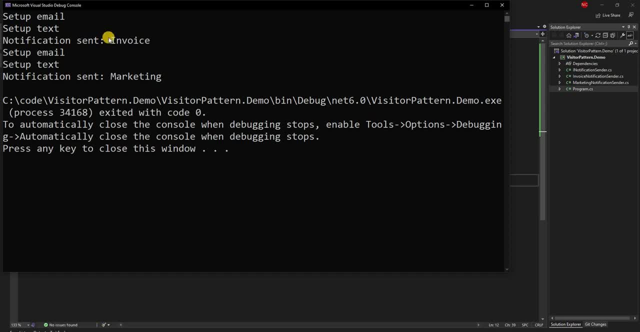 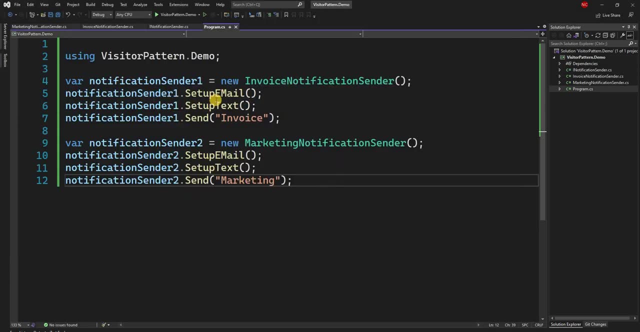 to show that, yeah, we are setting up email, setting up text, then sending a notification to invoice and then thing for marketing. Now, the biggest problem with this implementation is that if we have to send, if we decide that now we want to send a notification through a web socket or we want to, 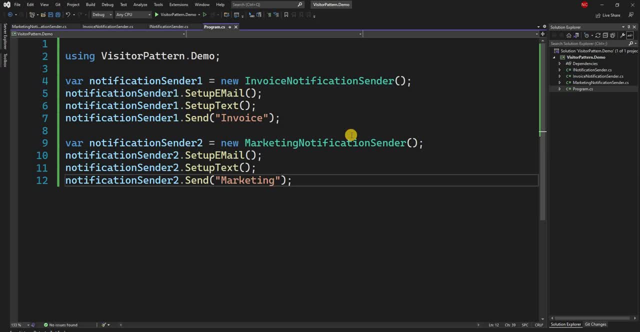 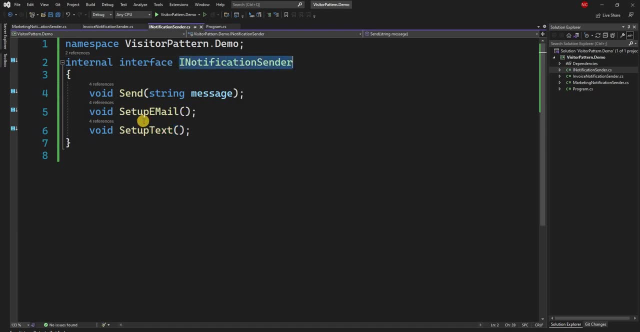 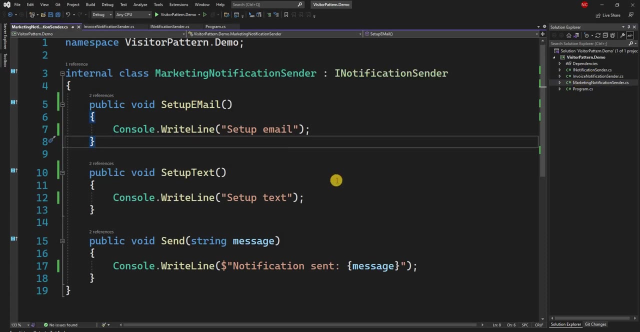 also add a notification to the mobile applications using Firebase notification, Then our implementation of the notification sender needs to be updated to add two new methods here, and then we'll have to go and update each of the class. So this is where the visitor pattern comes in. 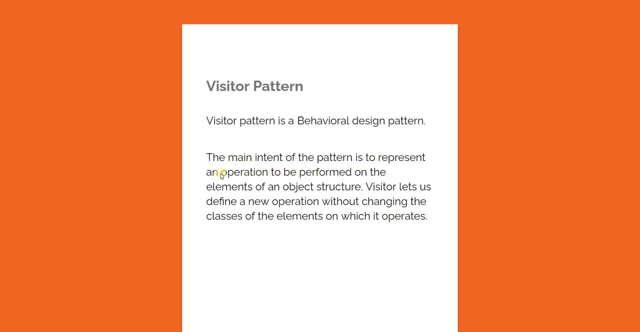 As you remember, based on the intent- Now let's look back into the intent, then it will be clearer this time- Is that to represent an operation to be performed on the elements of an object structure. So the operation that we are trying to perform on the element of the 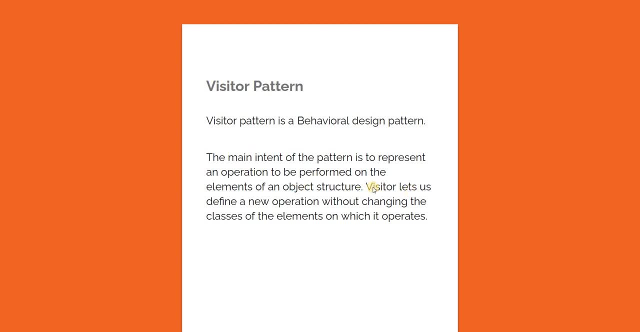 object structure is to set up email or set up text, and then we can have a visitor that lets us define an object structure. The key thing here is to provide an object structure so that the define a new operation without changing the classes of the elements in which it operates. 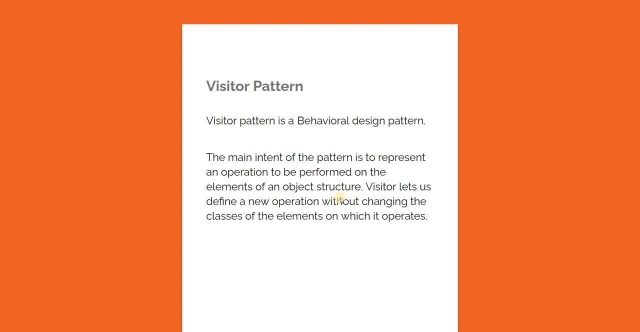 Meaning, if we take the setup of email and text out of this class and define it in visitor class, let's the visitor define the operation, in which case, even if we want to have a new type of notification protocol, it is not going to change our implementation of notification sender itself. 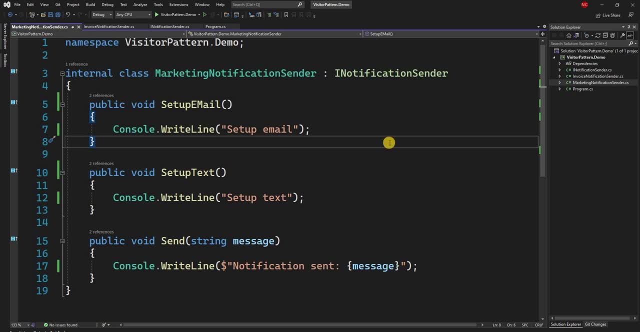 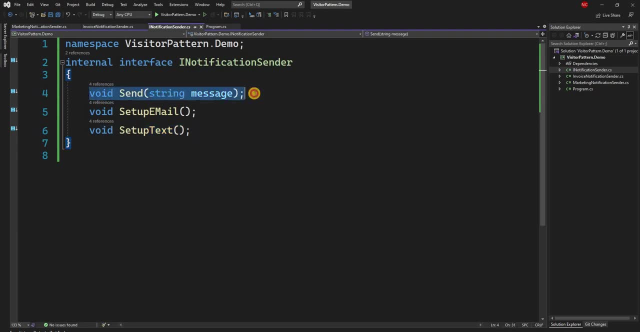 So now let's go back and try to refactor this implementation. So, at a primary goal, what we want to do is we want to keep the notification for sending notification and we want to give the setup to the visitor. So for that we have to accept the visitor. So let's define a method. 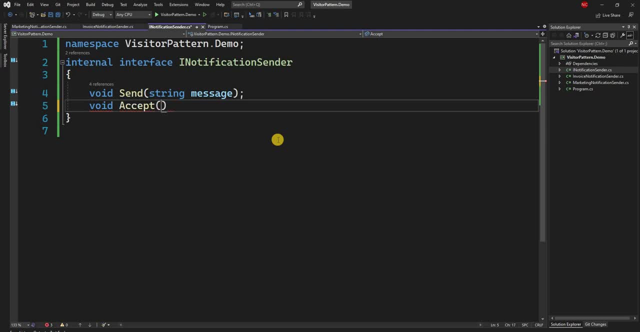 called void accept, and it is going to accept a new interface called visitor iVisitor. So let's define this interface and the visitor itself is going to have a single method, void visit, and here the visitor is going to take inotification sender as a input parameter. 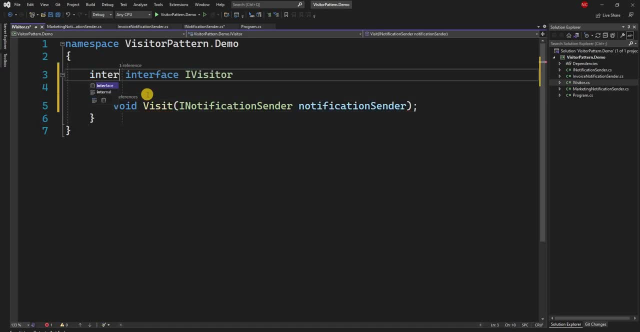 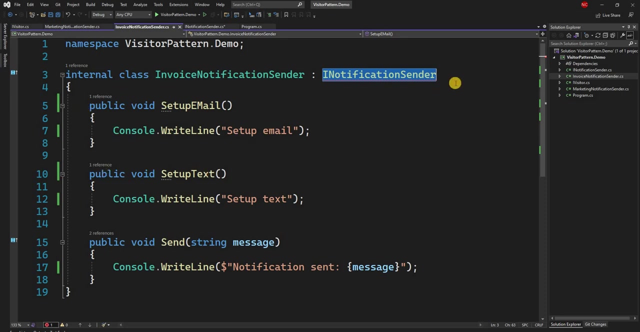 and let's make it as internal. So now we define the visitor interface. Next, what we are going to do is now: from the invoice sender and marketing sender, the implementation is going to change, So the setup email and setup text does not exist anymore. 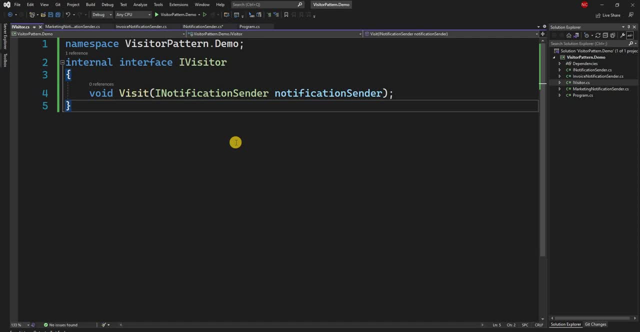 These responsibilities will be taken care by the visitor. So how will we define the visitor? So, for visitor, what we can do is we can define a class call, and I'm going to define the class right here, because it's a small class, so I can define it here. 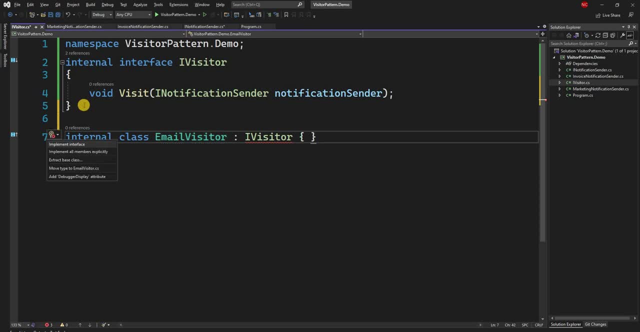 So we can have an email visitor, and the email visitor is going to basically set up the email protocol on the inotification sender. But for here I'm just going to copy and paste this consolewriteline considering: this is what is going to set up. 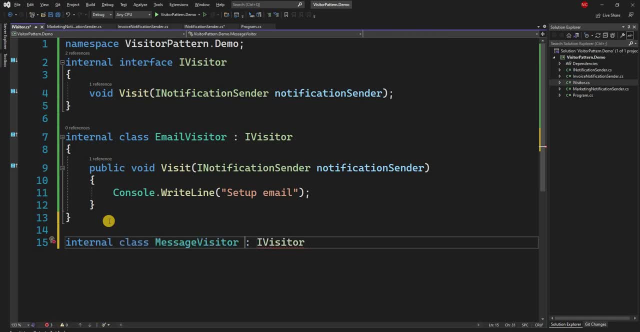 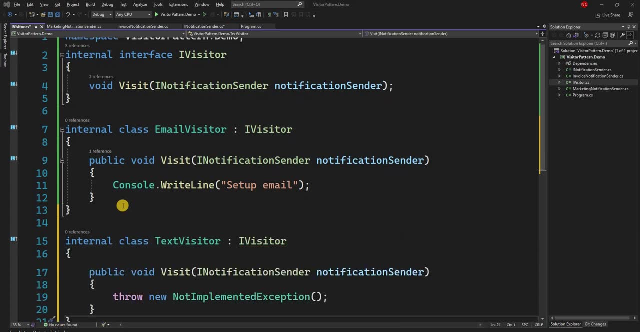 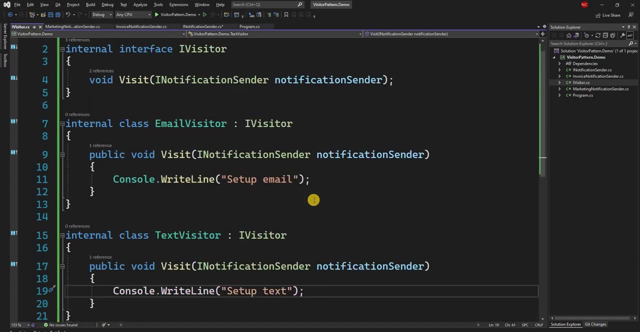 And similarly, we can have another class, Another class called text visitor, And the text visitor is going to do the same thing, it is just going to do a consolewriteline. So, as you can see, by implementing the visitor we moved the implementation of setting up. 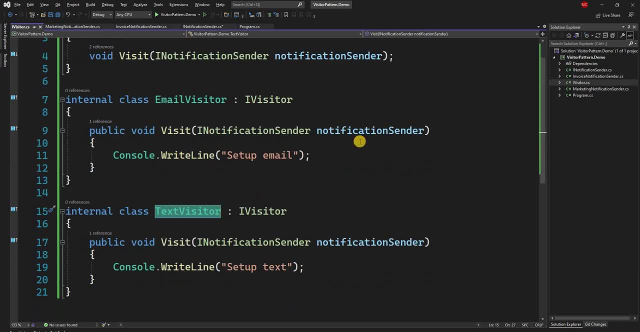 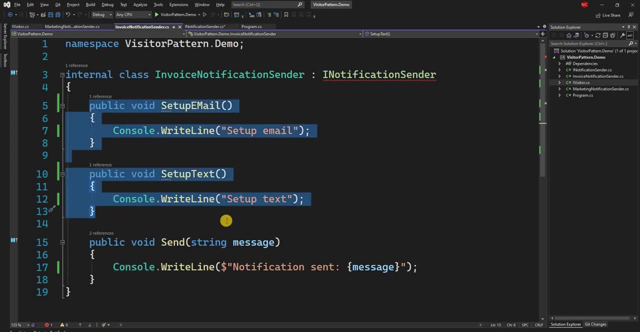 the email as well as text protocol outside of the notification class or the notification sender class. So at this point, we can get rid of these two methods. These are not required anymore. And here in the accept method, what we are going to do is we are just going to call the. 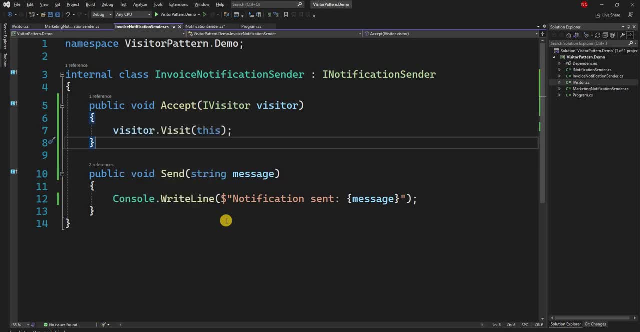 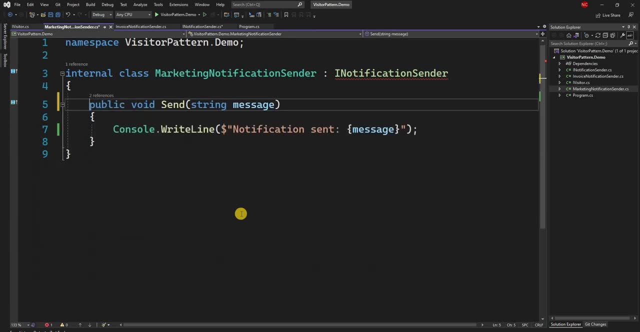 visitorvisit and we are going to pass the current class into it. Similarly, for marketing notification sender, we are going to have the exact same implementation where we are going to say visitorvisit of this. So this completely changed the landscape Of how this is going to work. 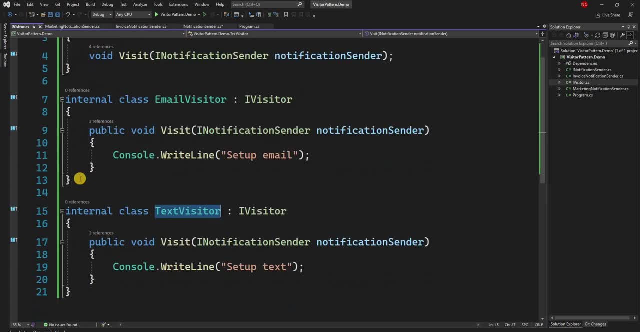 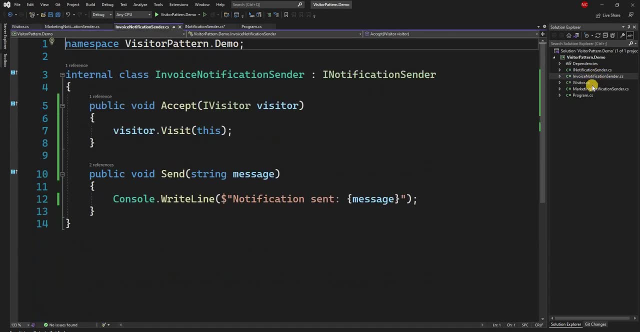 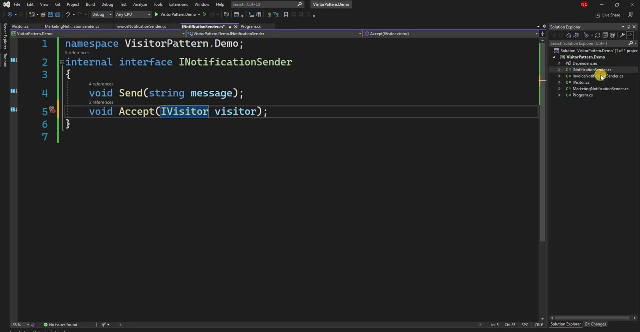 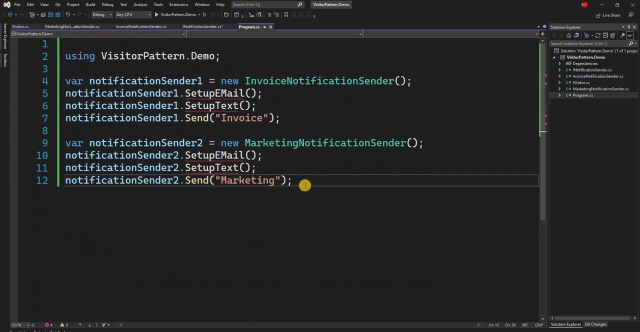 Now, as you can see, for the visitor, just like email or text, we can easily add new visitors in the future and it is not going to impact the invoice notification sender or marketing notification sender or the core interface of notification sender, because this association between the notification sender and the visitor will be managed by the caller or the setup. 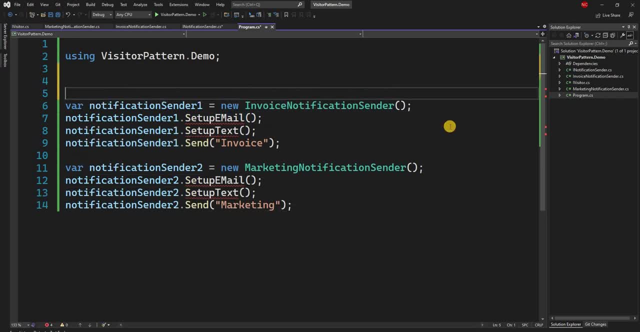 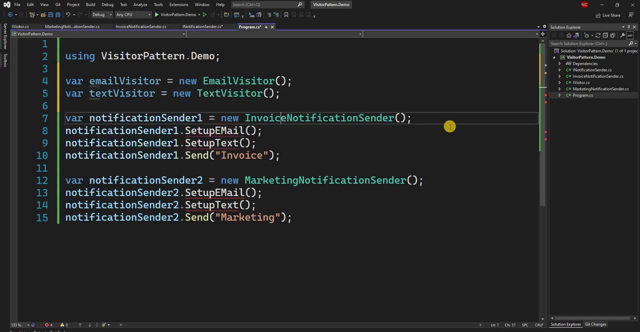 function. So here now, what we can do is first we will declare email visitor is equal to new email visitor and var text visitor equal to text visitor. and here what we can do is we can accept email visitor, Accept text visitor, And so that's it. 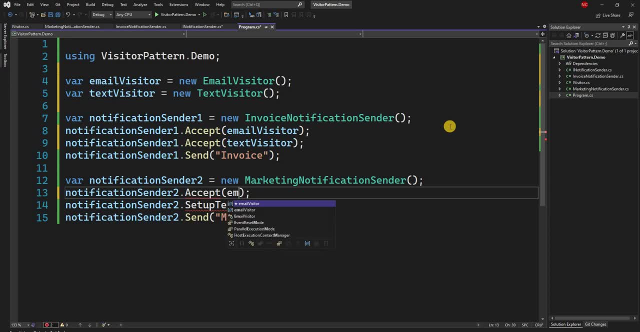 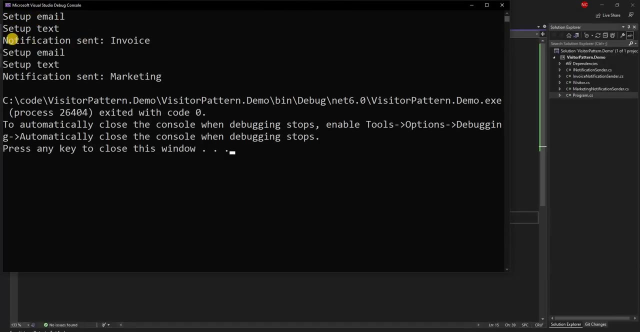 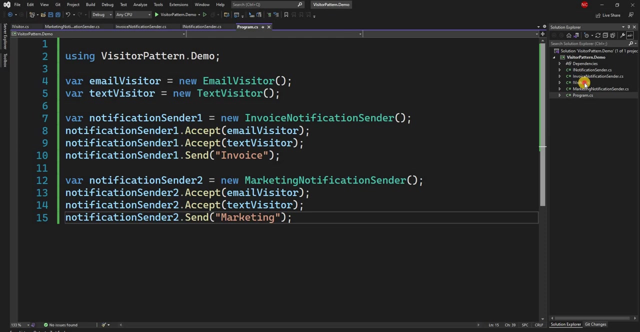 Thank you very much. same thing here, except email visitor, except text visitor. and now, if we run this function, it is going to behave exactly same as the previous implementation: setup email, setup text send notification. setup email, setup text, send notification. now, if we decide that we need. 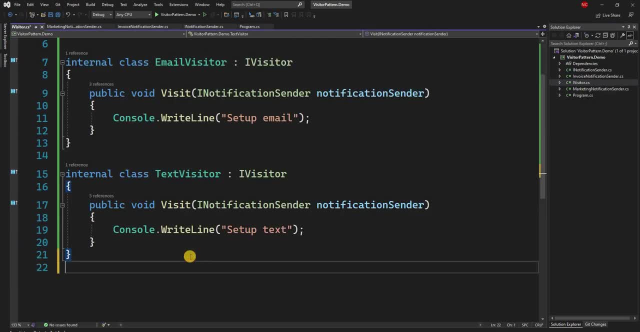 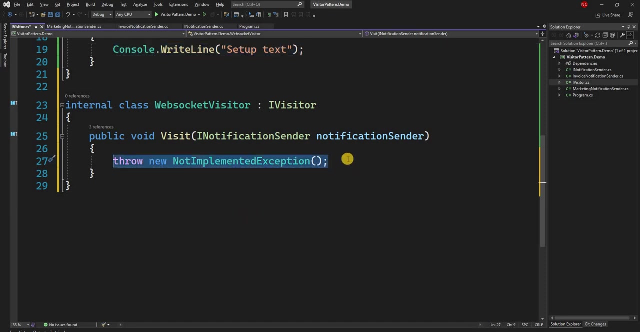 another type of visitor, let's say a web socket visitor. so we can simply go ahead and create an new class web socket visitor which is going to implement the i visitor and in the implementation here we can just do a consolewrite line for the time being to show how it works but, as you can understand, ultimately for all the visitor. 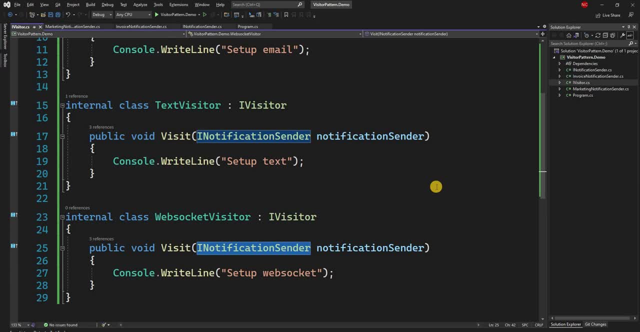 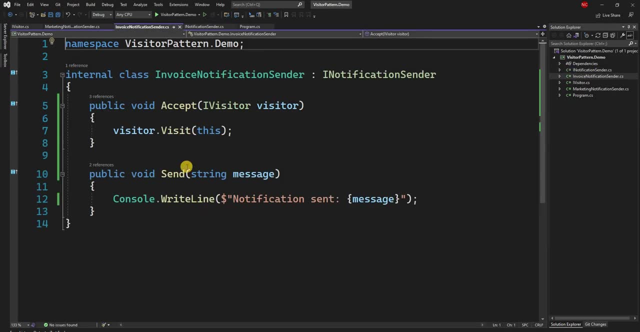 i notification center class will be used to set up the notification protocol for that notification, and this is what is ultimately going to be used while a notification is sent. what type of protocol? but i have not detailed everything here because that's a full-fledged implementation. so now we created 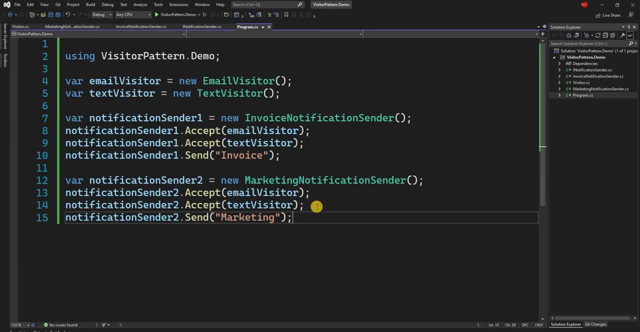 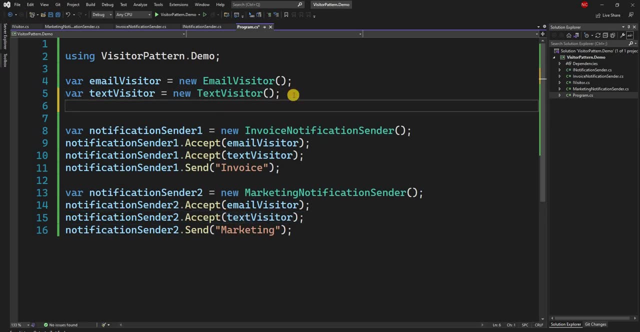 a web socket visitor and let's say, for the marketing notification, we want the web socket also to be sending notifications. so all we have to do is here we have to declare var web socket visitor equal to new web socket visitor. and here what we can do is we can. 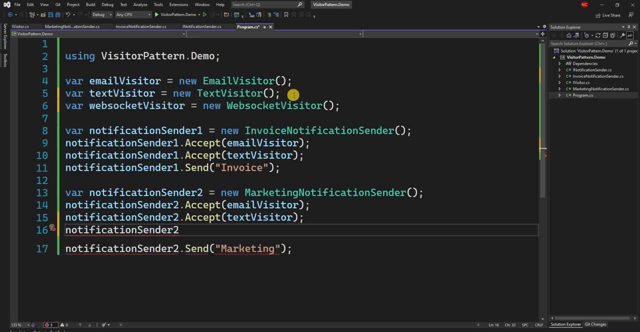 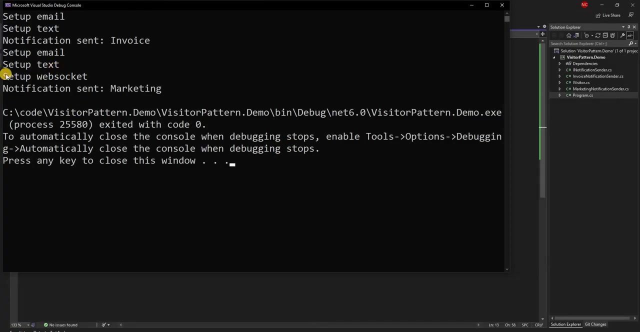 say, for the notification sender to dot accept, and here we can say web socket visitor, and now the marketing notification sender is going to send notification through email text and web socket visitor. and, as you can see, we did not have to make any change to the marketing notification sender for achieving a new type of protocol for sending notification and as